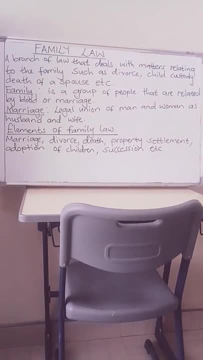 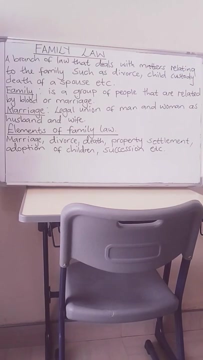 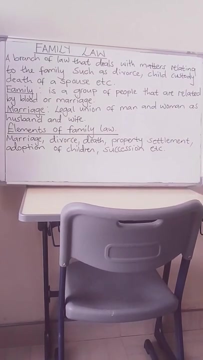 Okay so family law is actually defined as a branch of law that deals with matters relating to the family, such as divorce, child custody, death and etc. etc. Okay so let's just define family law in civic education. This topic here encompasses family in marriage. It actually 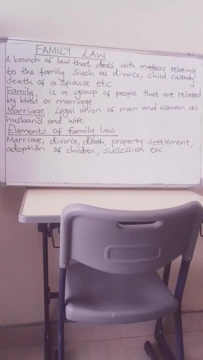 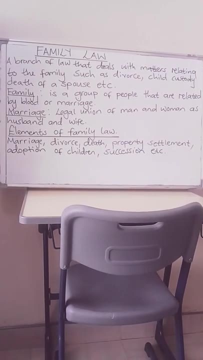 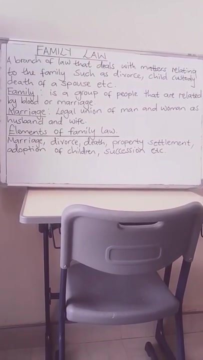 talks about family as well as marriage. So when you see family law in civic education, just think of family as well as marriage. So let's just describe the two. Okay, so we are saying family is a group of people that are related by blood or by marriage. Okay, family is a group of 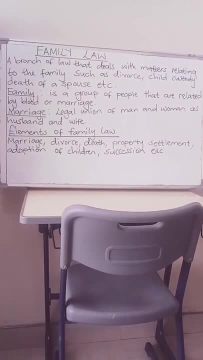 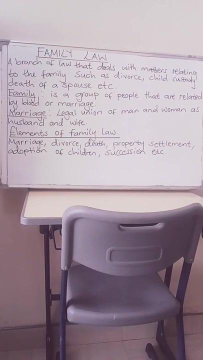 people that are related by blood or by marriage. Okay, so what is marriage? Marriage, we are saying is a legal union of man and woman as husband and wife. Okay, so it's very important for me to describe these terms to you. I need to define these terms so as to make the work easier for you. 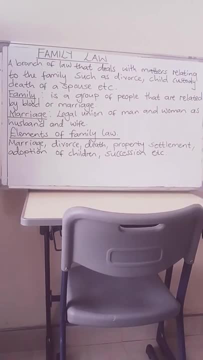 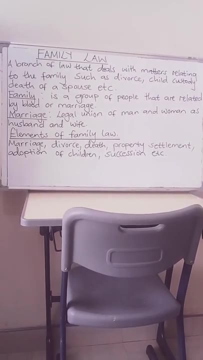 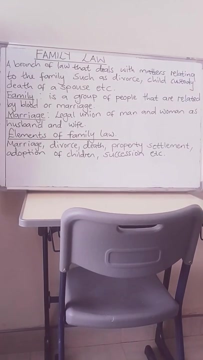 Okay, so let's talk about elements of family, Elements of family law. Okay, so we have marriage. marriage is actually an element of family. Okay, we have divorce When two people that are married legally separate for good, okay, or forever, that is a divorce. We have death. Death is actually an. 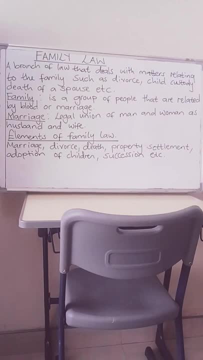 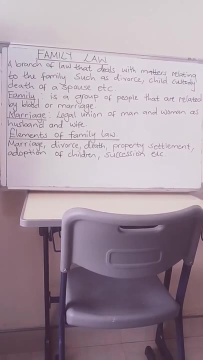 element everywhere in society. There's death in friendships, There's death in marriage, There's death in relationships. There's death everywhere. Okay, so we have property set element. Okay, that's within the family property settlement. We have adoption of children- Some. 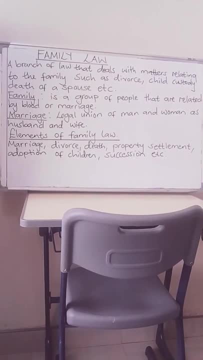 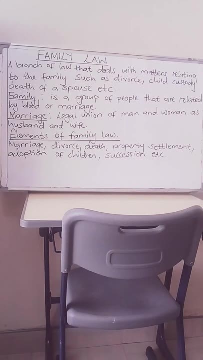 marriages, as well as families, adopt children, We have succession, etc. etc. Now, when it comes to succession, there are a lot of things that people succeed. Okay, so you can succeed money from. it can be your father, your uncle or your guardian. Okay, when they die, you take up.